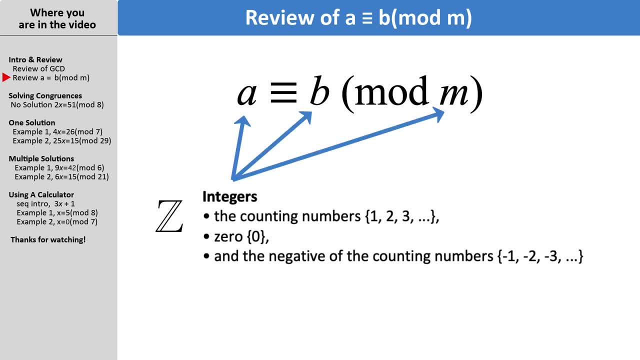 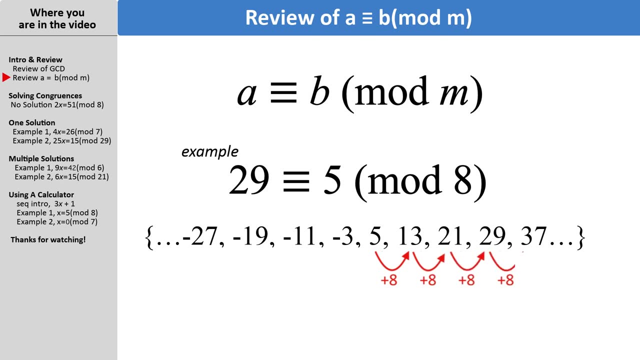 where a and b and m are integers. That means no decimals and no fractions. An example of a congruence with working numbers would be: 29 is congruent to 5 mod 8.. This is what we call a least residue system mod 8.. It's a set of integers that are a multiple of 8.. 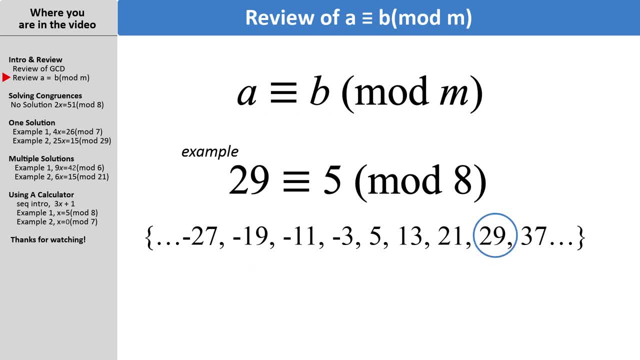 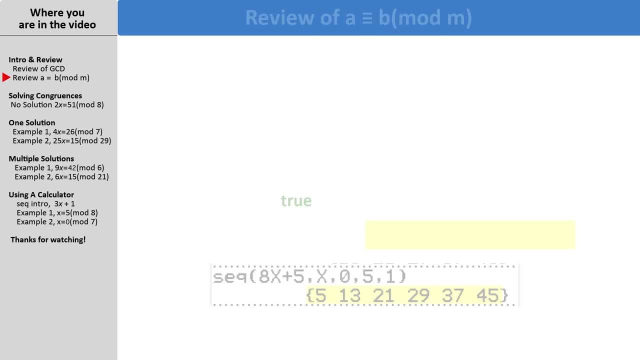 By inspection you can see 29 is here, so the congruence is true. We will see how to quickly make these on a calculator. after the examples of how to solve, We're going to look at three outcomes of the solving process. Number one: the case that 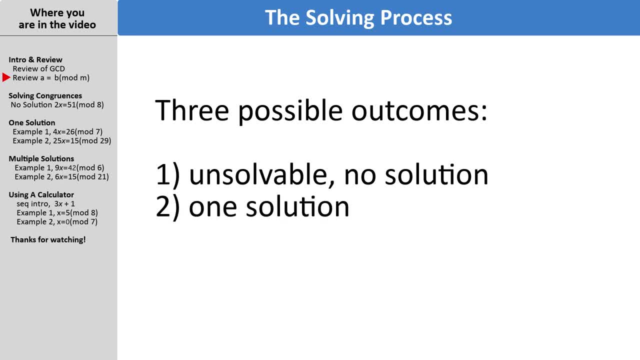 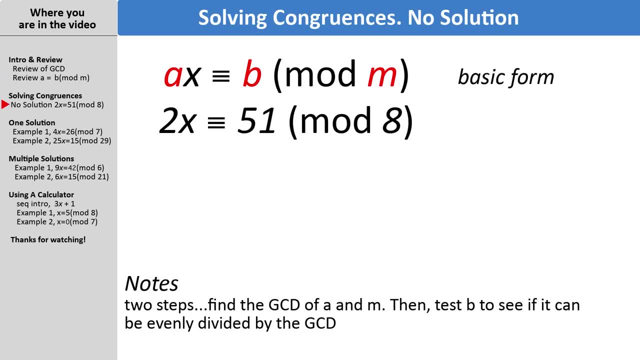 is unsolvable. Number two, the case where there is a single solution And number three, the case where there is more than one solution. Let's start with the unsolvable case. When you get one of these, they're easy And the 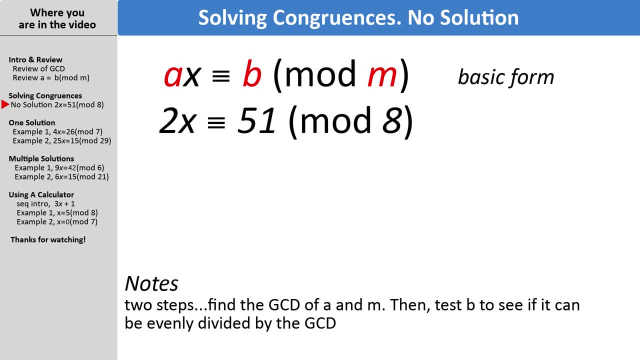 test is simple. There's only two steps. Here's the form. a is congruent to b mod m. First, find the GCD of a and m. In this example, the greatest common divisor of 2 and 8 is 2.. Fine, Next test if that evenly divides 51.. Nope, 2 does NOT divide 51. It would leave. 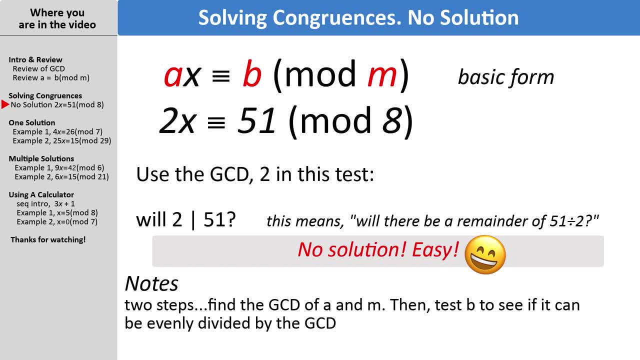 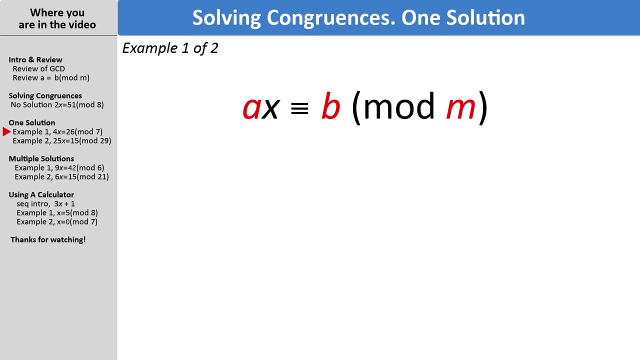 a remainder of 1.. So we can stop trying to solve this one. This is a no-go Case. number two: One solution: The greatest common divisor test we just saw is a necessary test when you begin solving any linear congruence. Let's take this one. 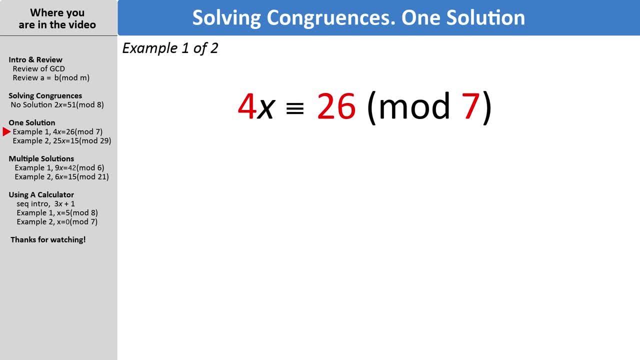 4x is congruent to 26 mod 7. start with finding the greatest common divisor with 4 and 7, which is 1, by the way, pro tip. if one of the numbers is prime, you know the GCD has to be 1. in this case, it's due to that 7, which is prime, since you've got a 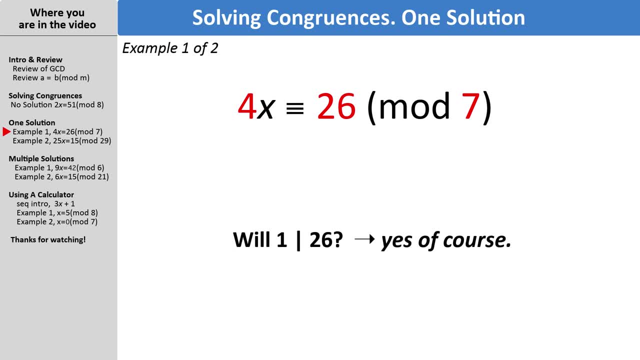 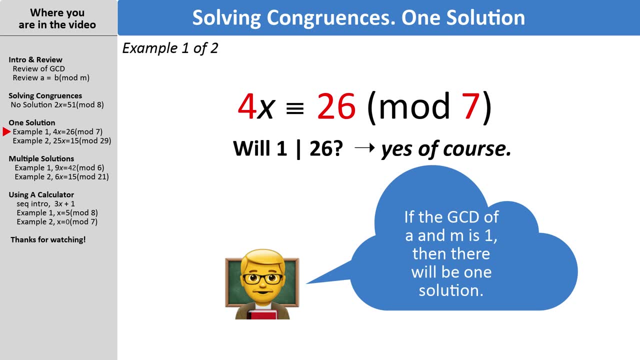 1, and the next step is to see if 26 can be divided by 1. yeah, of course, all integers can be divided by 1. so this is a point: you recognize that your linear congruence will have a single solution. so let's see how to get there. 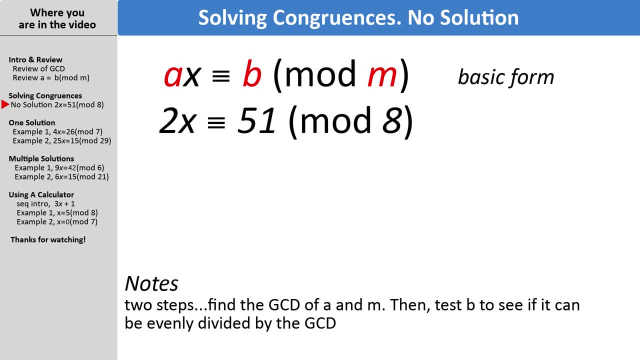 test is simple. There's only two steps. Here's the form. a is congruent to b mod m. First, find the GCD of a and m. In this example, the greatest common divisor of 2 and 8 is 2.. Fine, Next test if that evenly divides 51.. Nope, 2 does not divide 51. It would leave. 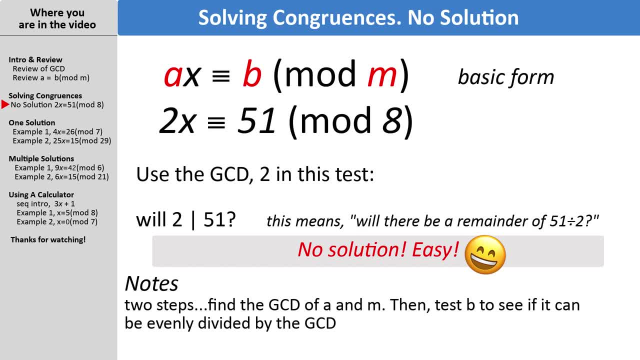 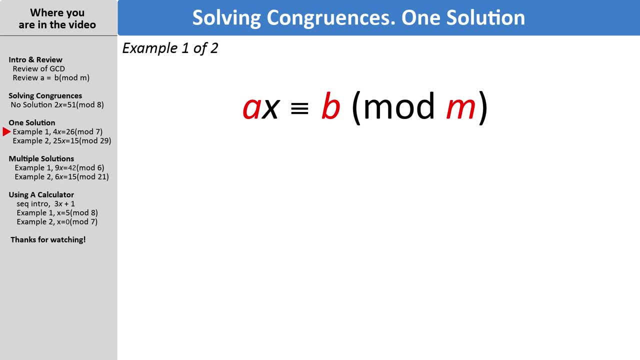 a remainder of 1, so we can stop trying to solve this one. This is a no-go Case. number two: one solution. The greatest common divisor test we just saw is a necessary test when you begin solving any linear congruence. Let's take this one. We've already got a two-division. 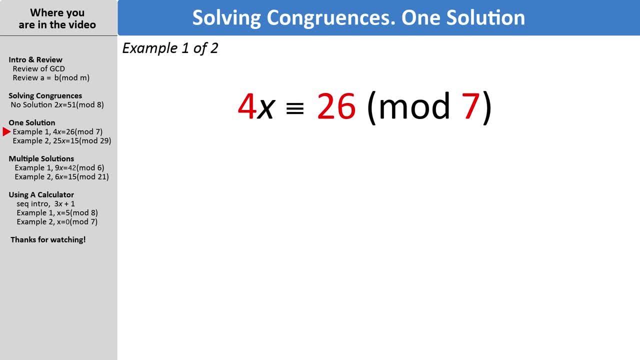 4x is congruent to 26 mod 7. start with finding the greatest common divisor with 4 and 7, which is 1, by the way, pro tip. if one of the numbers is prime, you know the GCD has to be 1. in this case, it's due to that 7, which is prime, since you've got a 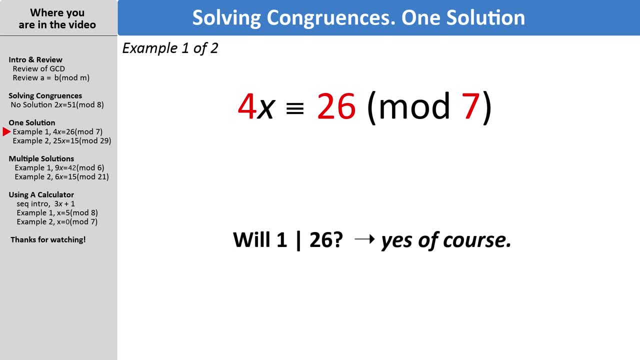 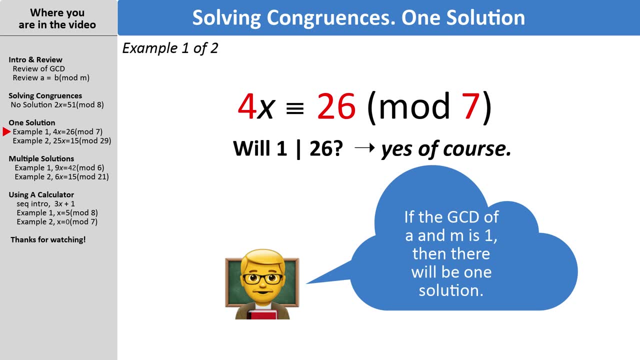 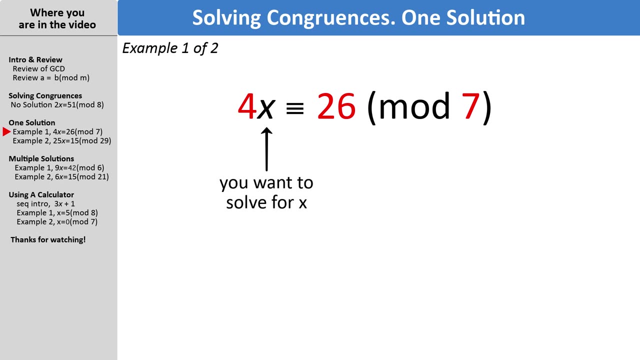 1, and the next step is to see if 26 can be divided by 1. yeah, of course, all integers can be divided by 1. so this is the point: you recognize that your linear congruence will have a single solution. so let's see how to get there. similar to: 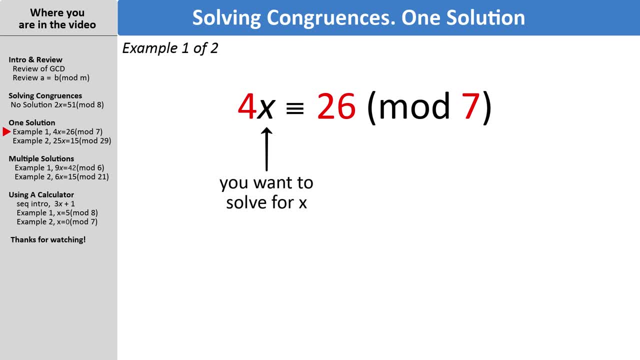 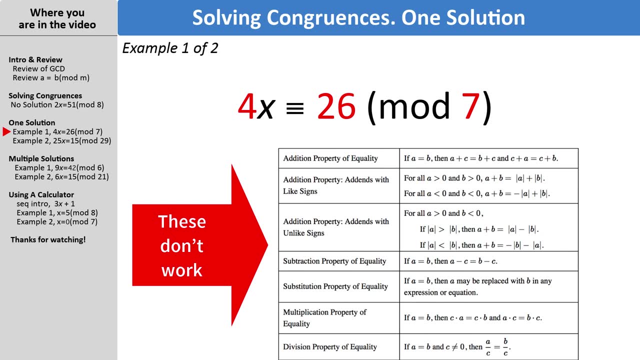 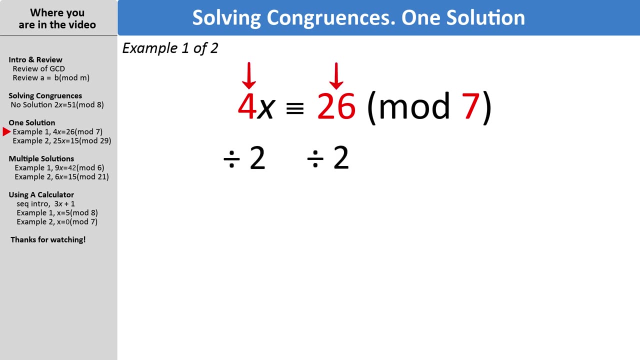 solving a linear equation. you want to isolate X. but don't be fooled: you don't have an equation and that's not an equal symbol. you can't simply subtract 26 or divide by 4. it doesn't work that way. so here's what you can do if both a and B 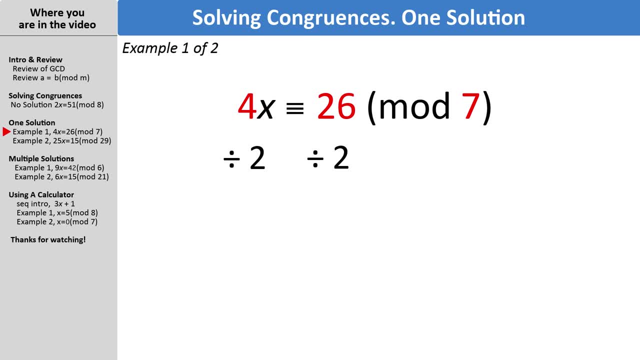 can be divided by 1 and the next step is to find the greatest common divisor with 26. then go ahead. for this example, 4 and 26 can be divided by 2 and you may rewrite the linear congruence as 2x is congruent to 13 mod 7. notice that we. 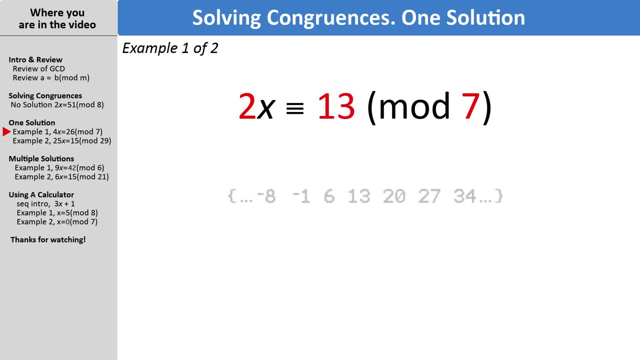 don't mess with that 7. now here's the fun part. look at the 7 and the 13 and consider the residues. ask yourself: can we add or subtract multiples of 7 to 13 and get it to be divisible by 2 and closer to 0?? 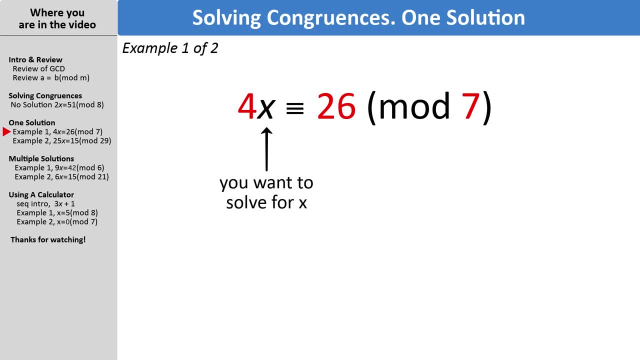 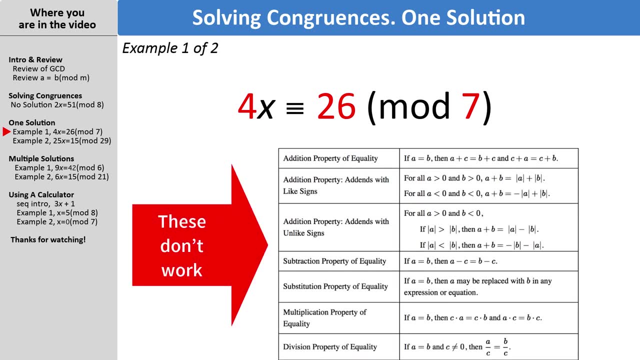 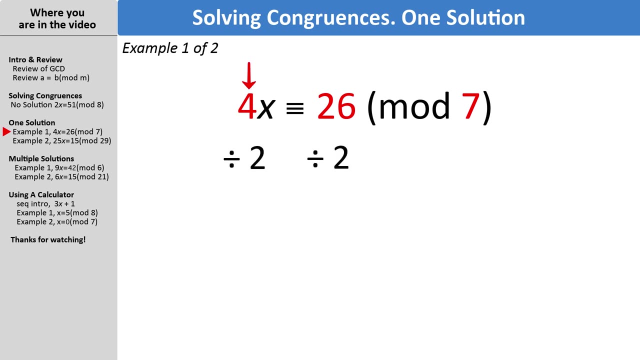 similar to solving a linear equation. you want to isolate X, but don't be fooled: you don't have an equation and that's not an equal symbol. you can't simply subtract 26 or divided by 4. it doesn't work that way. so here's what you can do if both a and b can be divided. 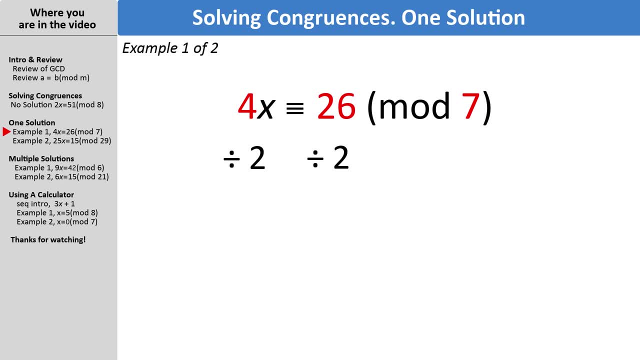 divided by an integer c. then go ahead. For this example, 4 and 26 can be divided by 2, and you may rewrite the linear congruence as 2x is congruent to 13 mod 7.. Notice that we don't. 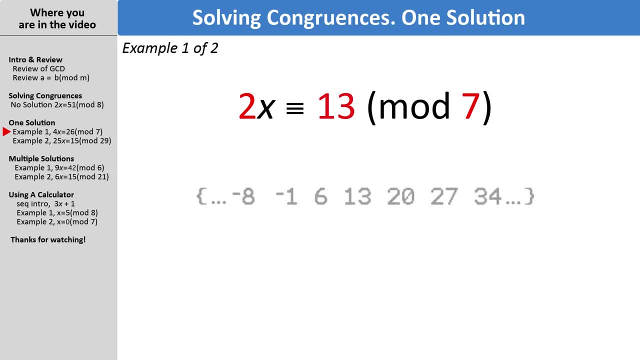 mess with that 7.. Now here's the fun part. Look at the 7 and the 13 and consider the residues. Ask yourself: can we add or subtract multiples of 7 to 13 and get it to be divisible by 2? and? 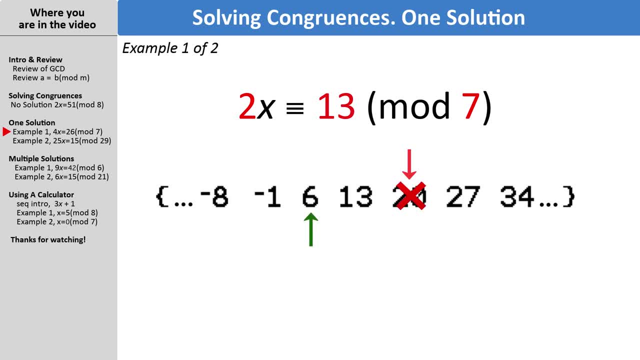 closer to 0?? Yes, it looks like we can use that 7 and walk it down to a 6 and then rewrite it to be 2x is congruent to 6 mod 7.. Great, Now dividing by 2 can be done and it becomes x is congruent. 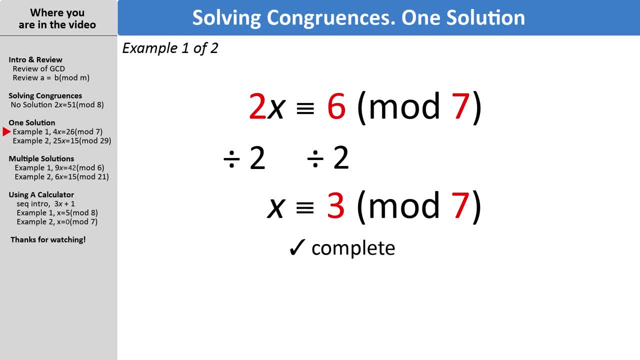 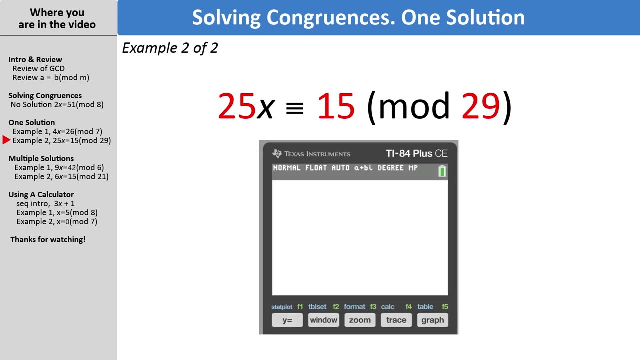 to 3 mod 7,, which is the final and only solution. Let's look at an additional example that is a bit more challenging. 25x is congruent to 15 mod 29.. The GCD of 25 and 29 is 1, and 15 can be divided. 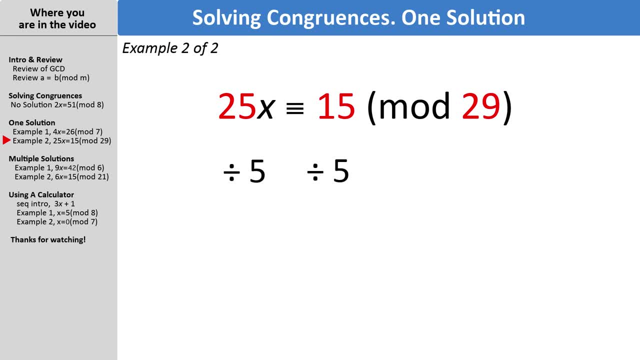 by 1,, of course, Start by dividing 25 and 15 by 1.. By the GCD, which is 5.. Having done that, we have: 5x is congruent to 3 mod 29, and it doesn't look. 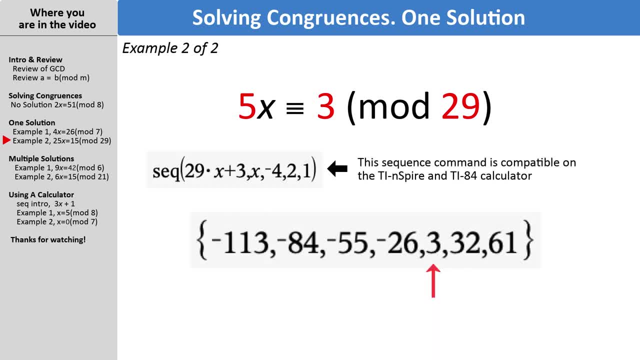 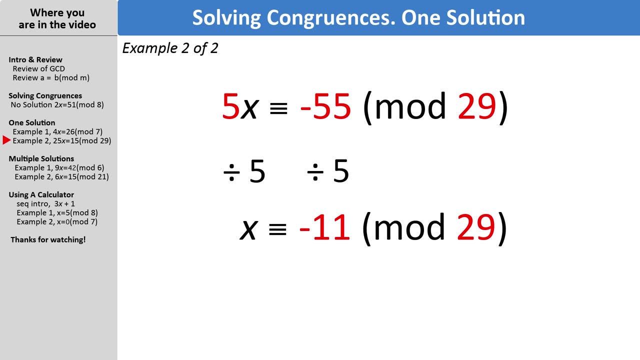 good, does it? Never fear, You can explore multiples of 29 that are negative and it looks like negative 55 will work out nicely. Dividing by 5, you get x is congruent to negative 11 mod 29.. 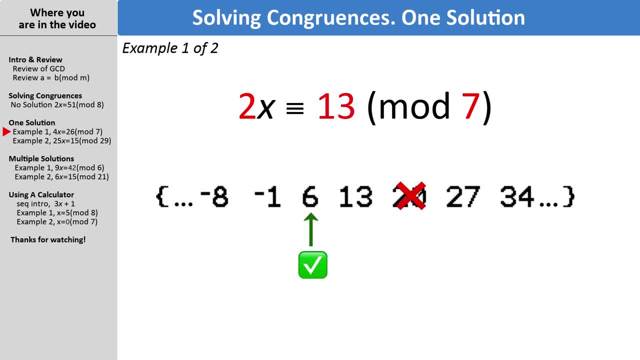 Yes, it looks like we can use that 7 and walk it down to a 6 and then rewrite it to be 2x is congruent to 6 mod 7.. Great, now dividing by 2 can be done and it becomes x is congruent to 3 mod 7,. 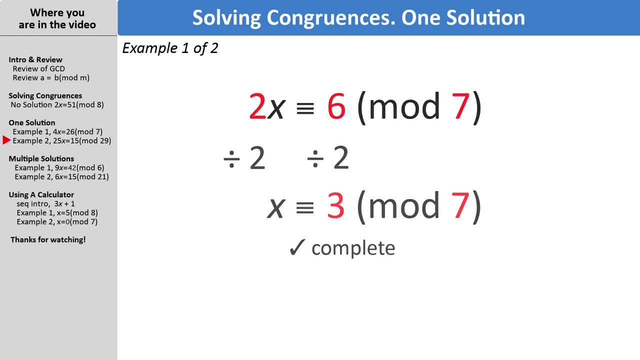 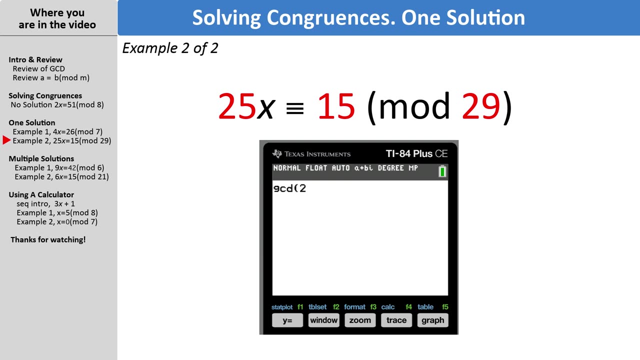 which is the final and only solution. Let's look at an additional example that is a bit more challenging. 25x is congruent to 15 mod 29.. The GCD of 25 and 29 is 1, and 15 can be divided by 1,, of course. 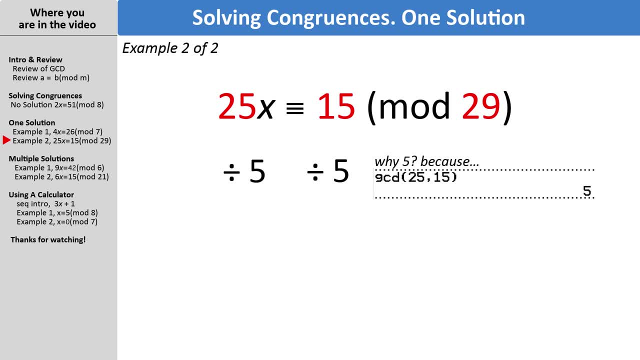 Start by dividing 25 and 15 by the GCD, which is 5.. Having done that, we have: 5x is congruent to 15 mod 29.. x is congruent to 3 mod 29.. And it doesn't look good, does it? 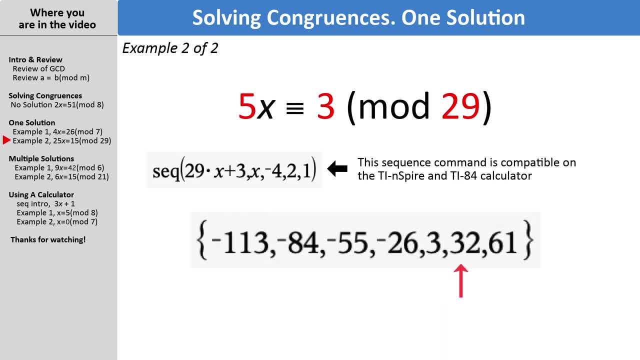 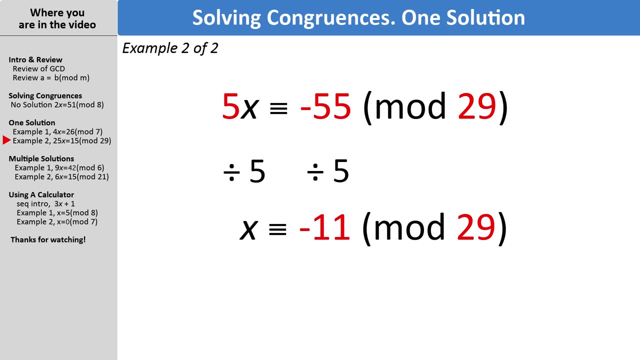 Never fear, You can explore multiples of 29 that are negative And it looks like negative 55 will work out nicely. Dividing by 5, you get x is congruent to negative 11 mod 29.. This is correct, but the final form of the answer should be: 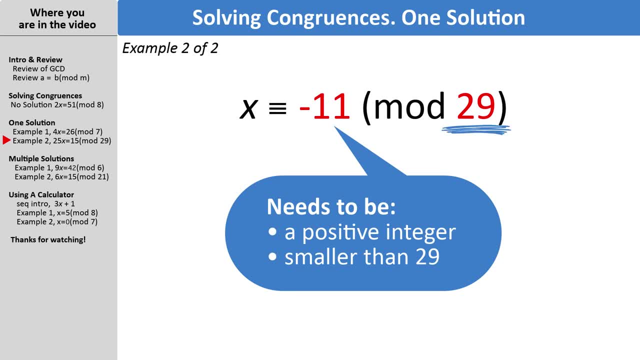 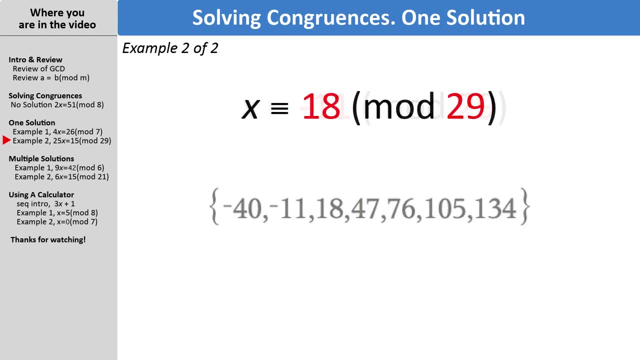 a value that is both positive and smaller than 29.. No problem here. Just add 29 to negative 11, and you get x is congruent to 18 mod 29. And you're done with this one Case number 3.. 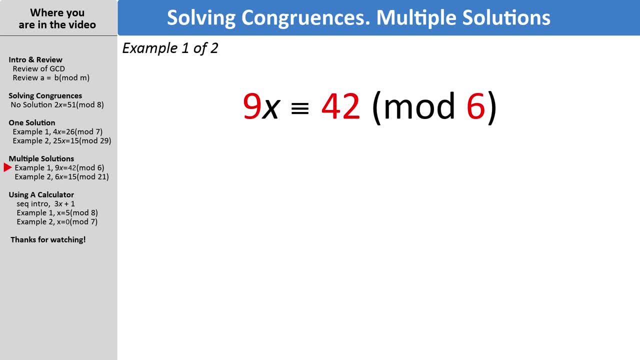 More than one solution. Buckle up. This one will have three solutions, Like before. let's check things out with the GCD test. The greatest common denominator of 9 and 6 is 3.. And a quick check: 42 is evenly divisible by 3.. 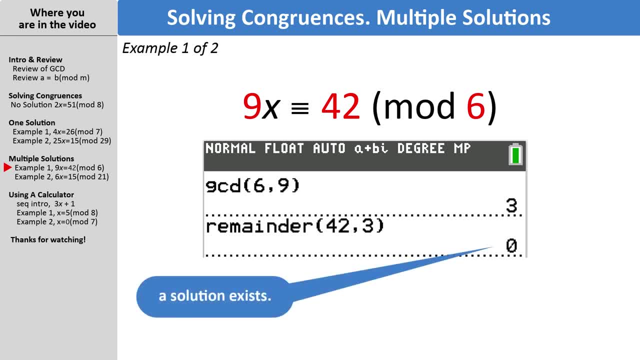 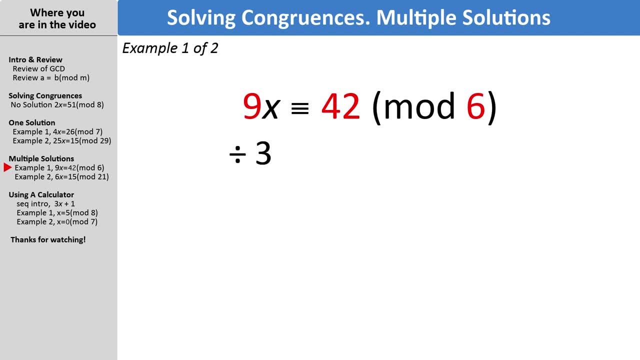 So we know two things. It has a solution, And there will be three solutions. This one has a nice property: Notice how every integer can be divided by 3. When you get to this situation, go ahead and do that. Dividing all by 3 simplifies. 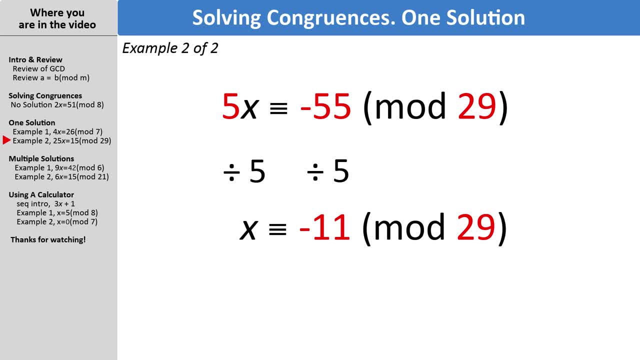 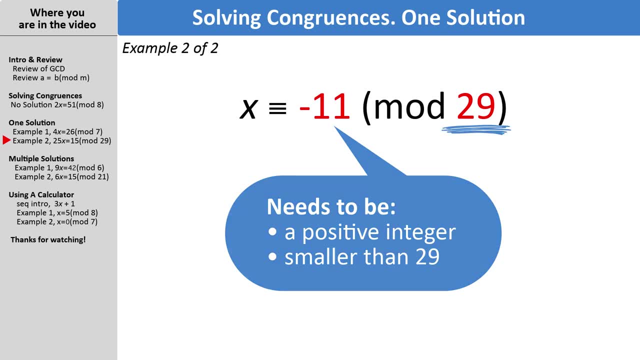 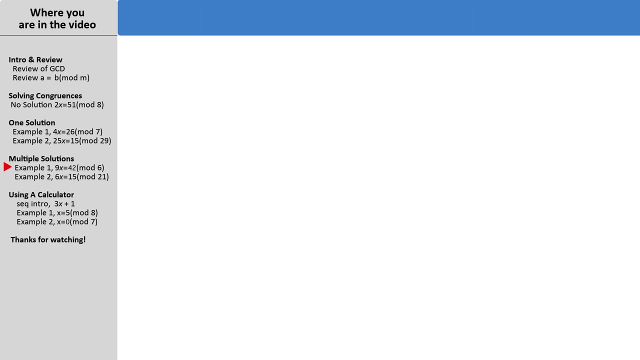 This is correct, but the final form of the answer should be a value that is both positive and smaller than 29.. No problem here. Just add 29 to negative 11, and you get. x is congruent to 18 mod 29, and you're done with this. one Case number three, more than one solution. Buckle up This. 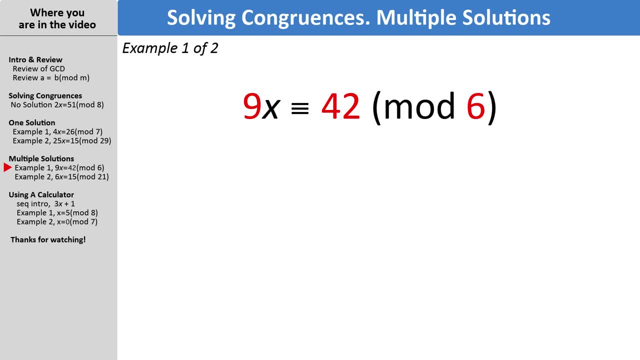 one will have three solutions, Like before. let's check things out with the GCD test. The greatest common denominator of 9 and 6 is 3, and a quick check: 42 is evenly divisible by 3,, so we know two. 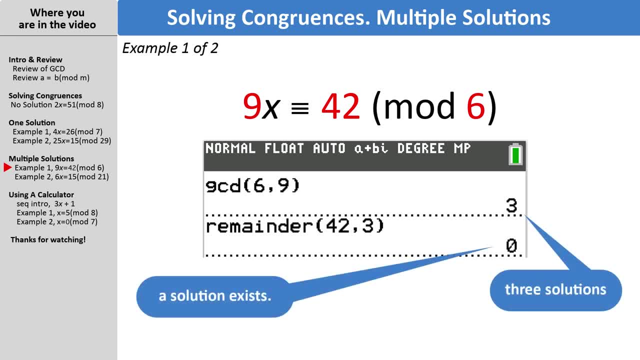 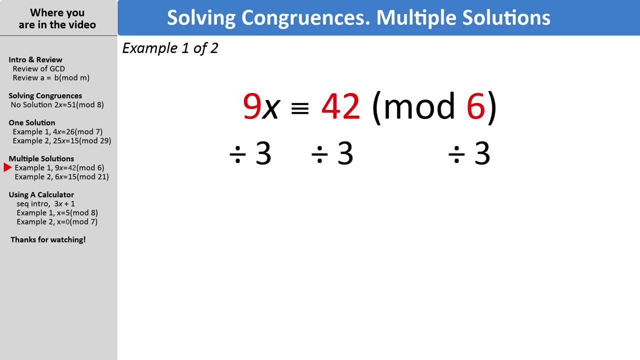 things. It has a solution and there will be three solutions. This one has a nice property: Notice how every integer can be divided by 3.. When you get to this one, you'll see that the integer is divided by 3.. In this situation, go ahead and do that. Dividing all by 3 simplifies to 3x is. 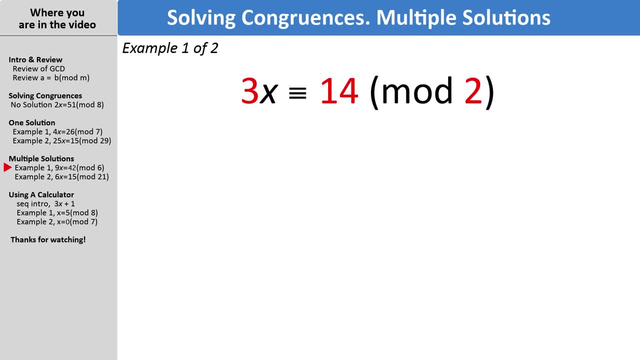 congruent to 14, mod 2.. Now let's see if we can walk down that 14 by multiples of 2 to get something that can be divided by 3.. You might be tempted to go with 12, but no, Remember, the idea is to get. 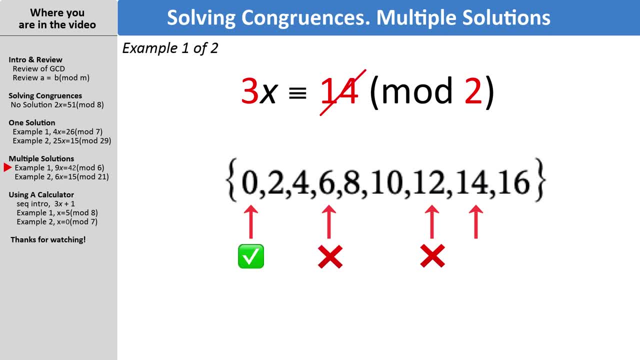 as close to zero as possible. Zero is kind of nice because zero can be divided by any number, so we definitely will go with zero. Write the simplified form as follows: X is congruent to zero mod 2, and this is called the solution in the least residue system. Let's not forget there. 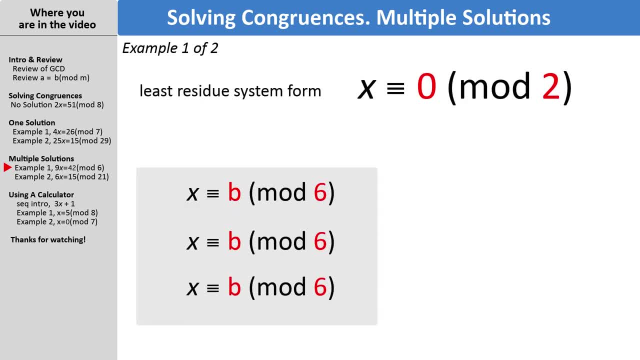 are three solutions, and here's how that works. We will find three values for B using a parametric method. We start by numbering from zero, one and two, and this can be the start of a table of values. The value B is generated by the equation: B is equal to 2t plus zero. starting with zero. 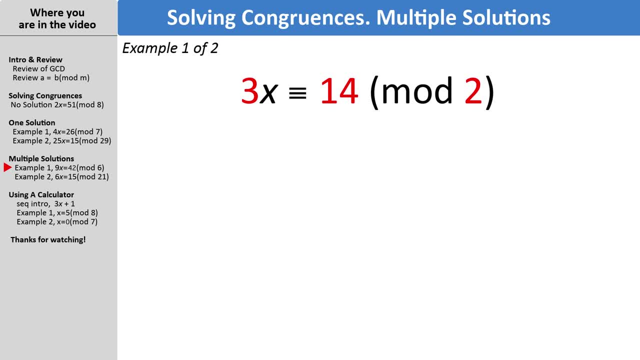 to 3x is congruent to 14 mod 2.. Now let's see if we can walk down that 14 by multiples of 2 to get something that can be divided by 3. You might be tempted to go with 12.. 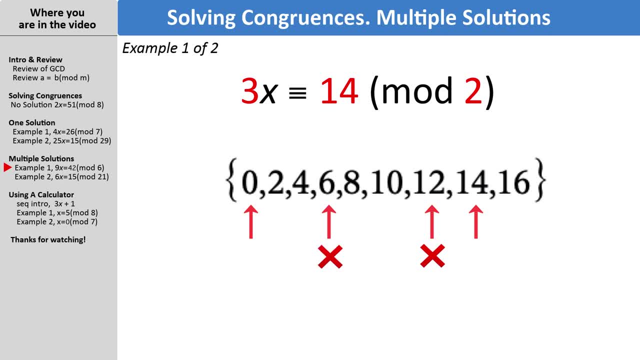 But no, Remember, the idea is to get as close to 0 as possible. 0 is kind of nice Because 0 can be divided by any number, So we definitely will go with 0.. Write the simplified form as follows: x is congruent to 0 mod 2.. 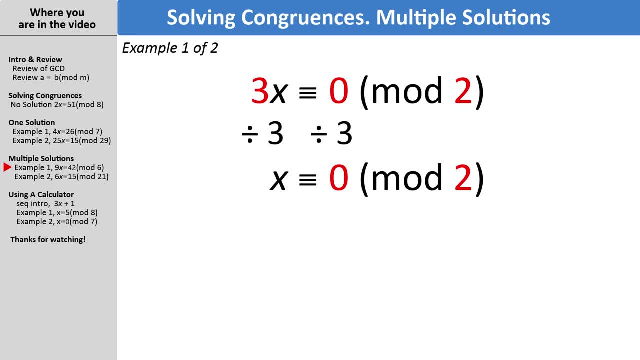 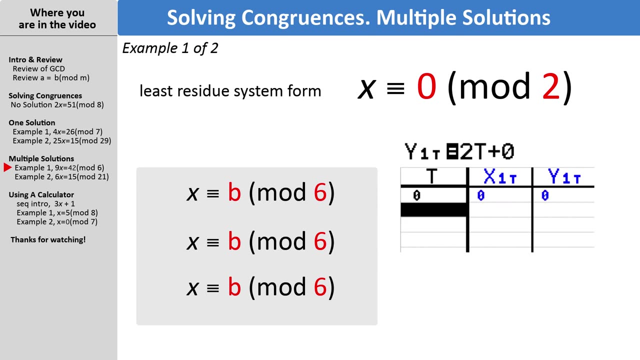 And this is called the solution in the least residue system. Let's not forget, there are three solutions And here's how that works. We will find three values for b using a parametric method. We start by numbering from 0,, 1, and 2.. 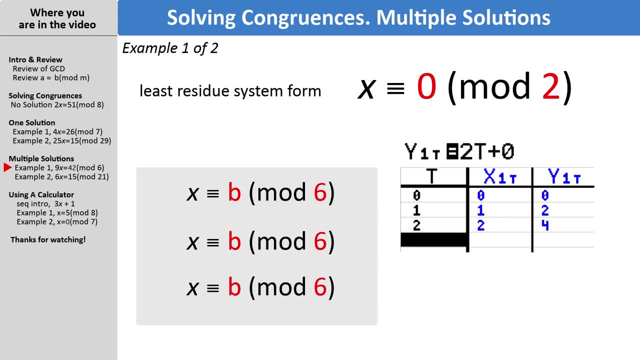 And this can be the start of a table of values. The value b is generated by the equation: b is equal to 2t plus 0.. Starting with 0. Then 2. Then 4.. The final solutions are written out with the original mod. 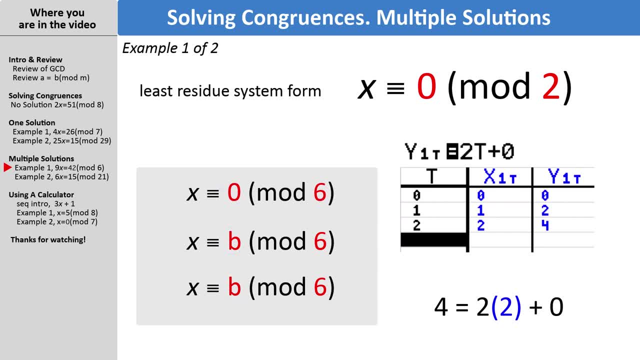 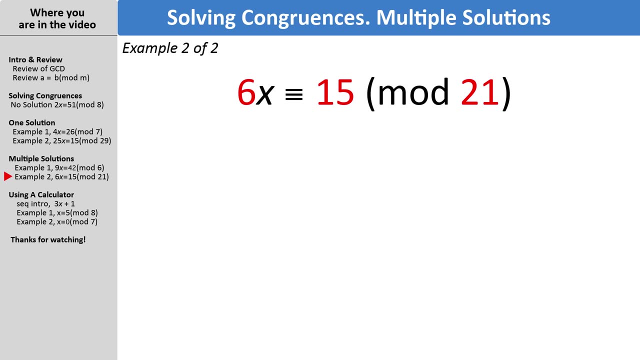 So we express them as: x is congruent to 0 mod 6,, 2 mod 6, and 4 mod 6.. Here's another example of a congruence with more than one solution: 6x is congruent to 15 mod 21.. 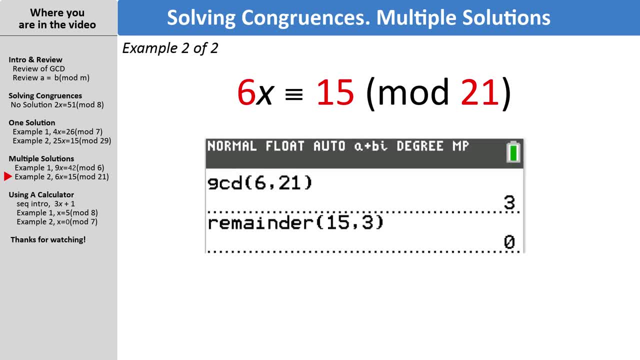 Let's move through this one a bit quicker. The GCD of 6 and 21 is 3.. And 15 is evenly divided by 3. So we are a go for finding three solutions. 6,, 15, and 21 are all divisible by 3.. 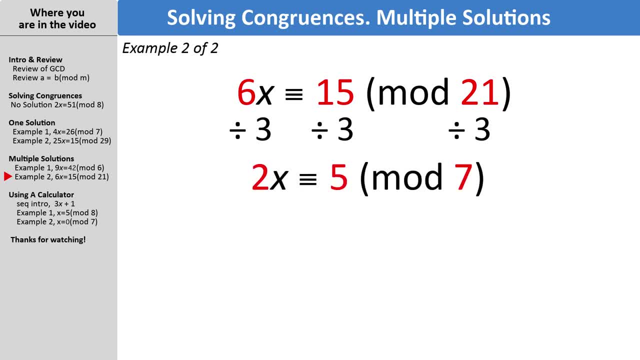 So we can simplify all by dividing by 3. And we get 2x is congruent to 5 mod 7.. So far, so good. We only need to somehow use multiples of 7 from 5 to find something that can be divided by 2.. 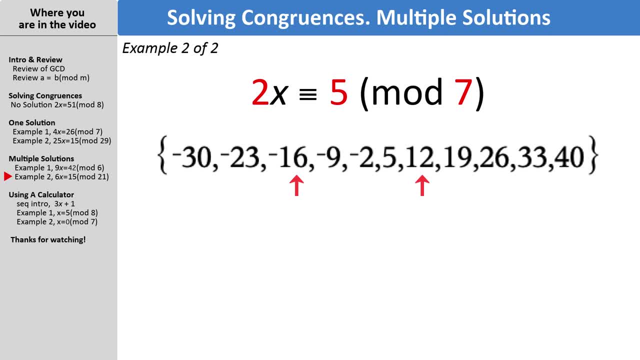 And we're home free. Looks like there are two possibilities: Negative 16 and 12.. One's up and one's down. Which to choose, It turns out you can choose either one of those. See if you choose negative 16,. 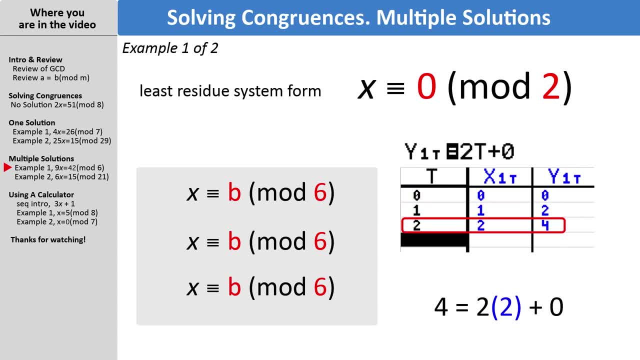 then two, then four. The final solutions are written out with the original mod, so we express them as: X is congruent to zero mod 6,, two mod 6, and four mod 6.. Here's another example of a congruent solution. 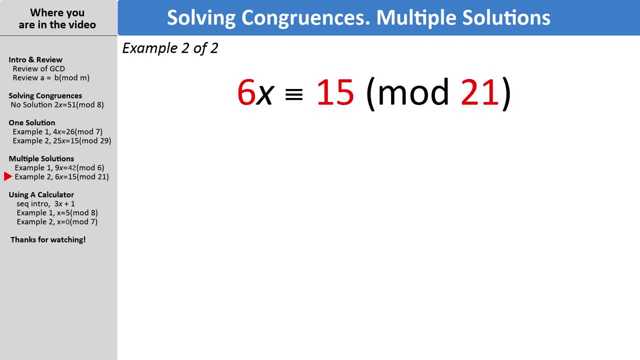 Let's move through this one a bit quicker. The GCD of 6 and 21 is 3, and 15 is evenly divided by 3, so we are a go for finding three solutions. 6,, 15, and 21 are all divisible by 3,. 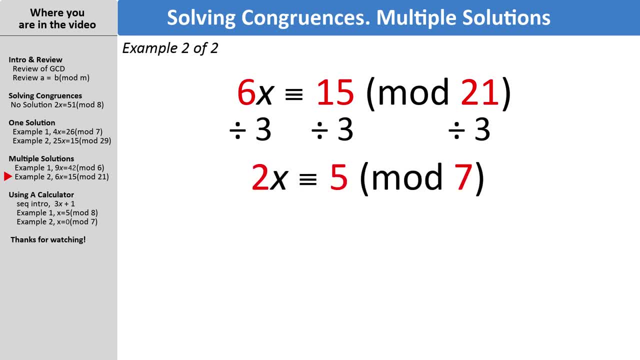 so we can simplify all by dividing by 3, and we get: 2x is congruent to 3, and 2x is congruent to 5 mod 7.. So far, so good. We only need to somehow use multiples of 7 from 5 to find something that. 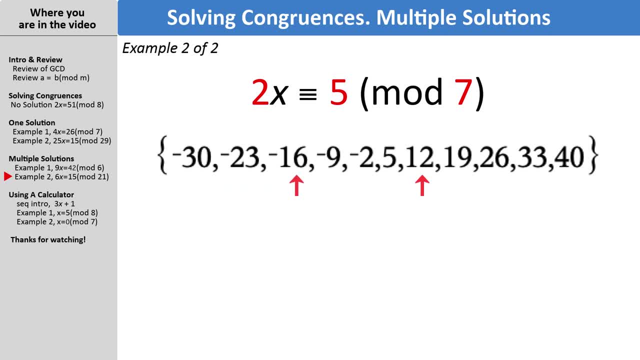 can be divided by 2, and we're home free. Looks like there are two possibilities: negative 16 and 12.. One's up and one's down. Which to choose, It turns out? you can choose either one of those. 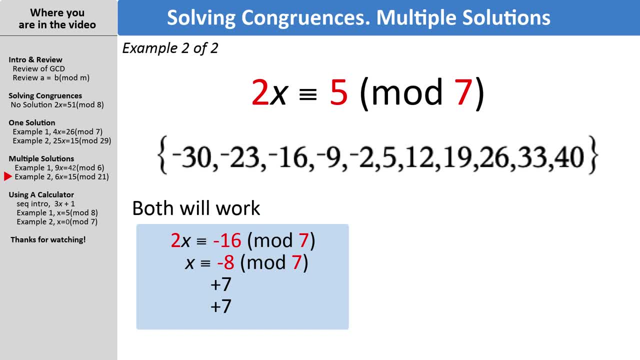 See: if you choose negative 16, you get. X is congruent to negative 8 mod 7.. The simplest form doesn't have a negative, so add multiples of 7 until you get a positive integer. X is congruent to 6 mod 7.. If you prefer to go up with multiples of 7,, 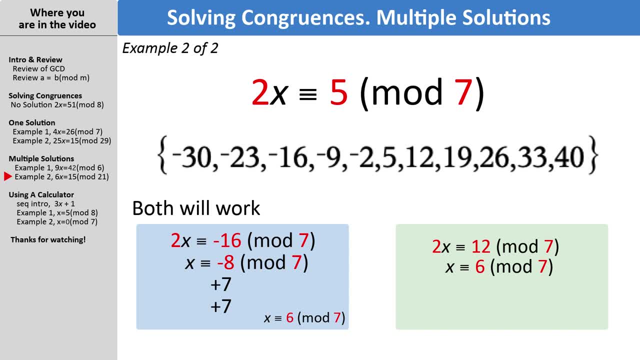 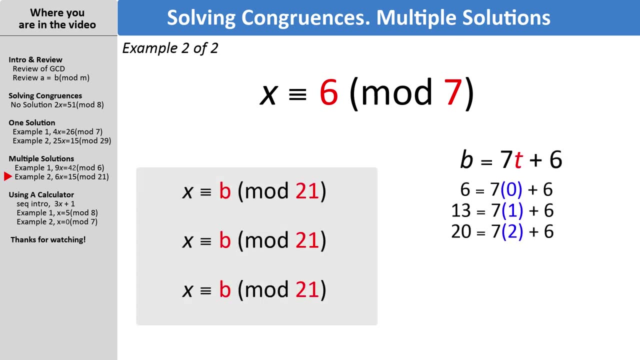 you get: 2x is congruent to 12 mod 7,, which simplifies to X is congruent to 6 mod 7.. So from here you need the three solutions. So we use the parametric form and a table Once again. 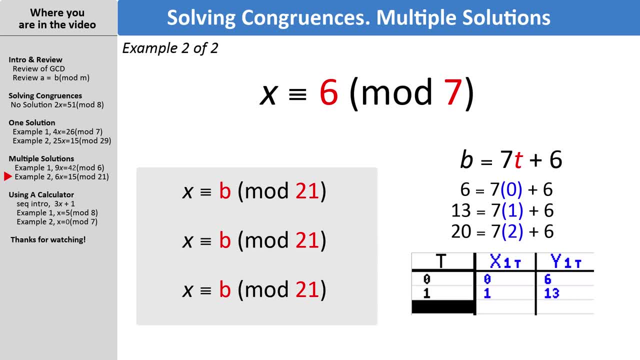 we count up from 0,, 1, and 2 in the table. Using the value of 0, the equation computes to 6,, 13, and 20.. Writing the solutions with the original mod of 21,. the answers are: X is congruent to 6. 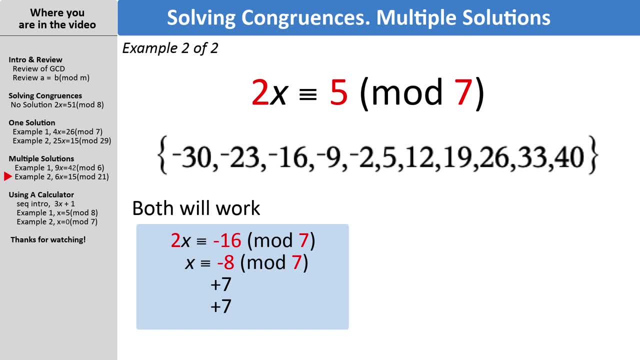 you get, x is congruent to negative 8. Mod 7. The simplest form doesn't have a negative, So add multiples of 7 until you get a positive integer. x is congruent to 6 mod 7.. If you prefer to go up with multiples of 7,, 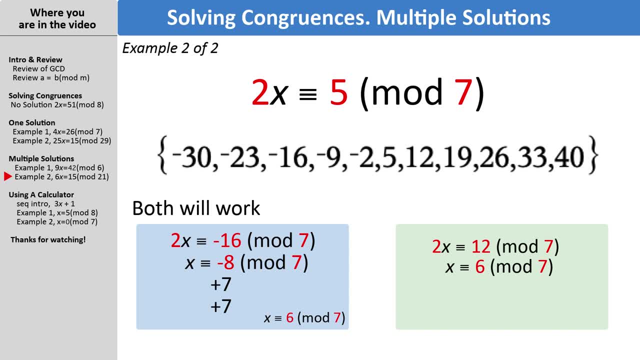 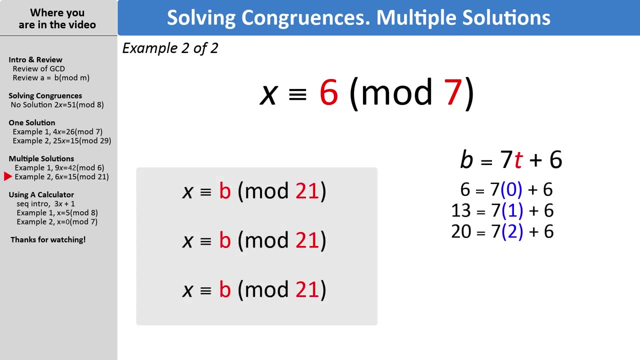 you get: 2x is congruent to 12 mod 7.. Which simplifies to x is congruent to 6 mod 7.. From here you need the three solutions. So we use the parametric form and a table. Once again, we count up from 0,, 1, and 2 in the table. 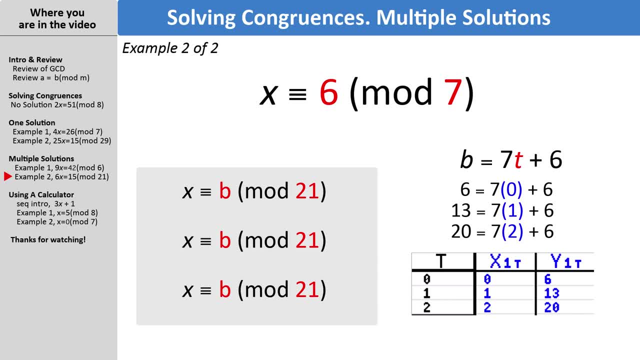 Using the value of 0,, the equation computes to 6,, 13, and 20.. Writing the solutions with the original mod of 21,. the answers are: x is congruent to 6 mod 21,, 13 mod 21, and 20 mod 21.. 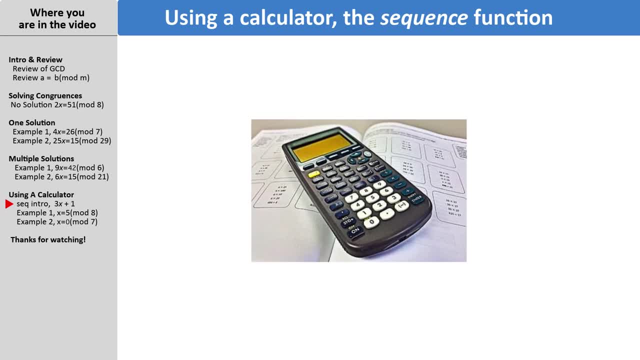 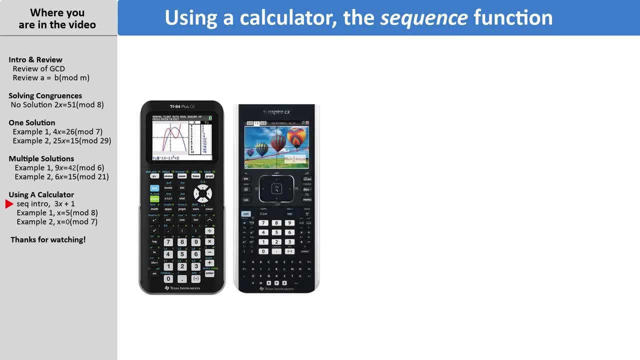 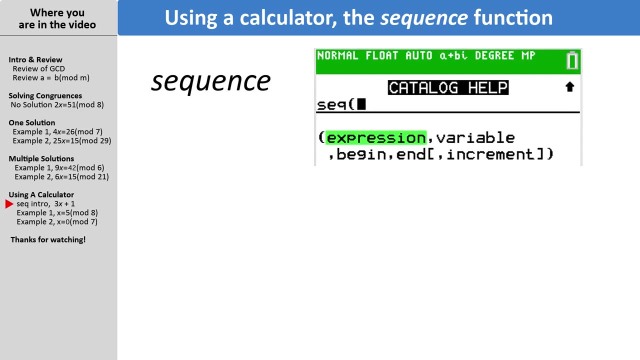 A final word on getting some help from a graphing calculator. The Texas Instruments TI-84 series and the TI-NSPIRE series have a handy function called sec, which means sequence, and will generate a list of values given an expression, a variable values for the low and high range and the step. 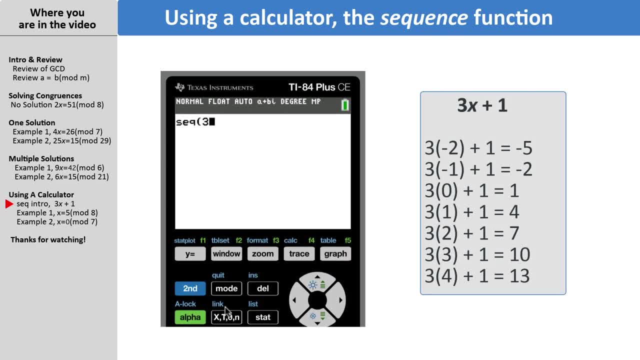 This is how to generate a simple list from the expression 3x plus 1, with a start of negative 2 and an ending value of 4, with a step of 1.. It's very handy for seeing least residue systems in some mod M. 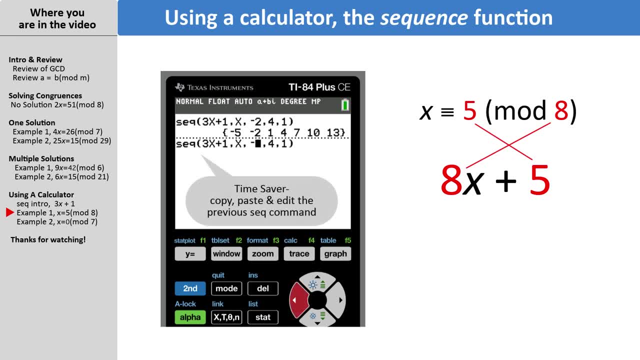 If we want to see, x is congruent to 5 mod 8,. you can code it in like this: sec: 8x plus 5, 8x plus 5, x negative, 4 to 4, with a step of 1,. 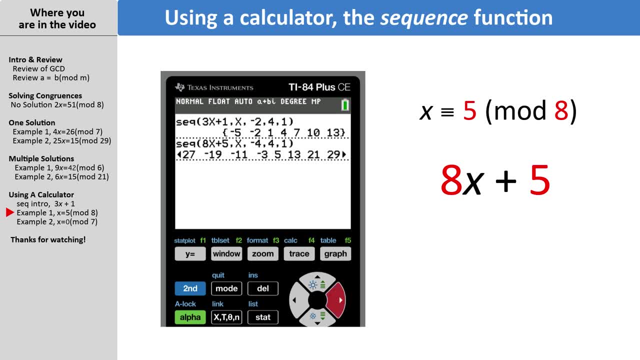 and you can see 8 values on either side of 5.. It's pretty nice. One more example: x is congruent to 0, mod 7.. It's coded as 7x plus 0, or simply 7x, since adding 0 doesn't do much.